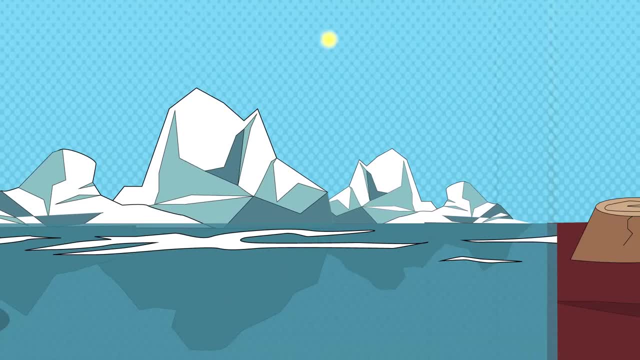 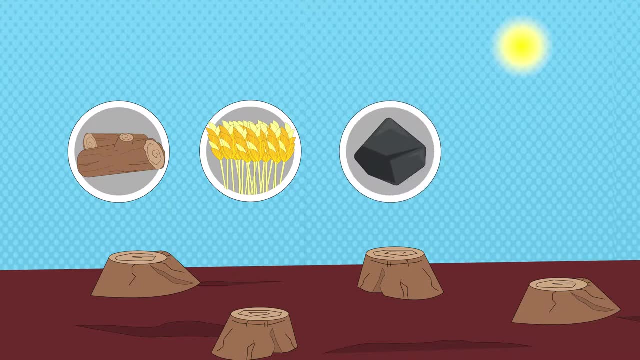 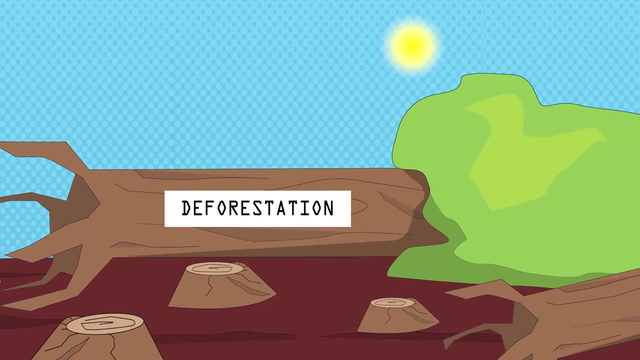 in its habitat and is an endangered species. Humans also require resources. Large areas of forest are cleared to make more room for agriculture or to mine minerals or for growing other resources like palm oil. The removal of trees is called deforestation and has an enormous impact on not only the local ecosystem but the entire planet. 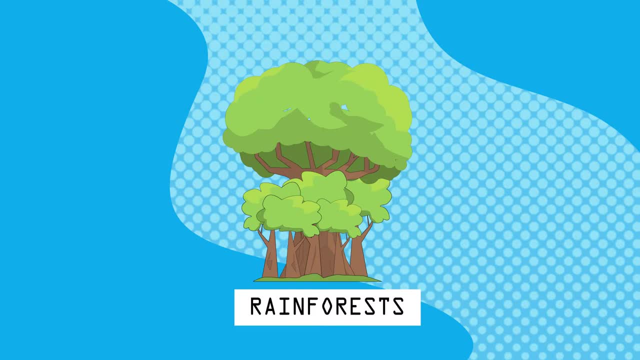 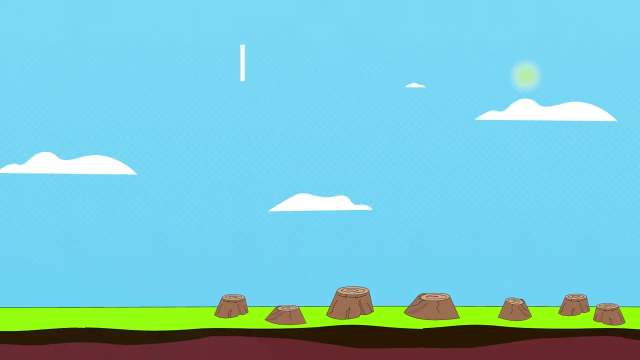 Ancient forests such as rainforests are unique ecosystems. They can support a high biodiversity and are home to species that can only live in that habitat. For example, in Borneo, rainforests are being cut down to make room for palm oil plantations. The species that live in the 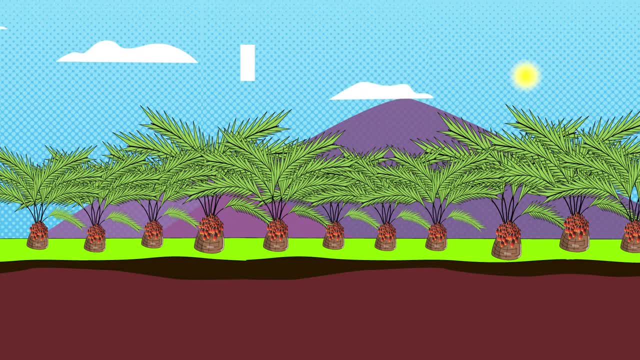 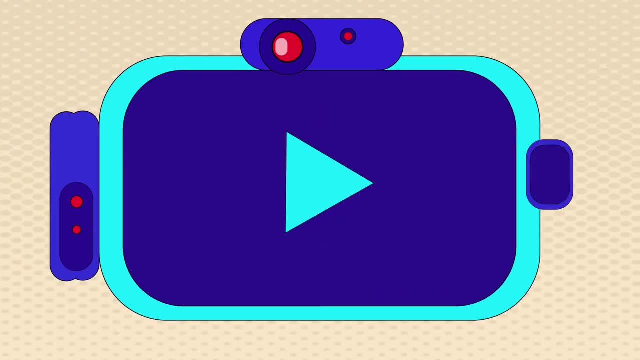 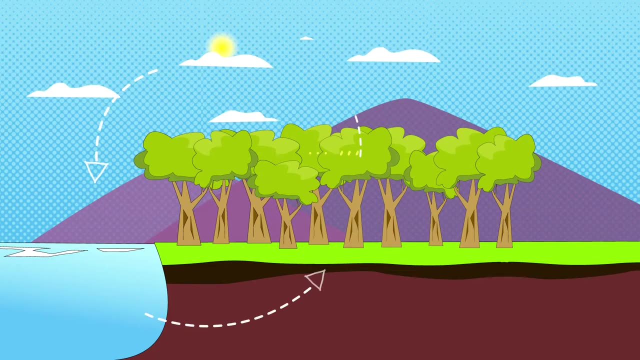 rainforests cannot survive in the plantations. They may not be able to find food or shelter like orangutans, who are an endangered species. You can find out more about endangered species and how conservation is helping them by watching this video. Forests provide services to the planet. They are important in the water cycle. They are 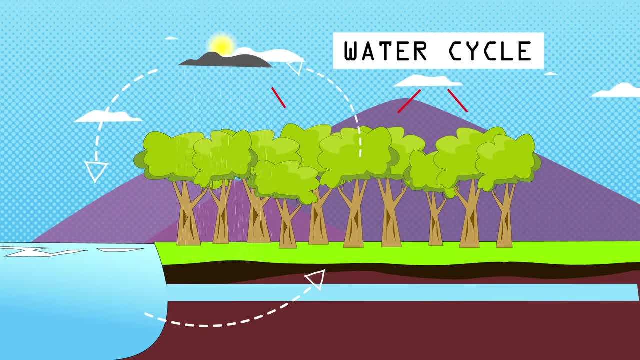 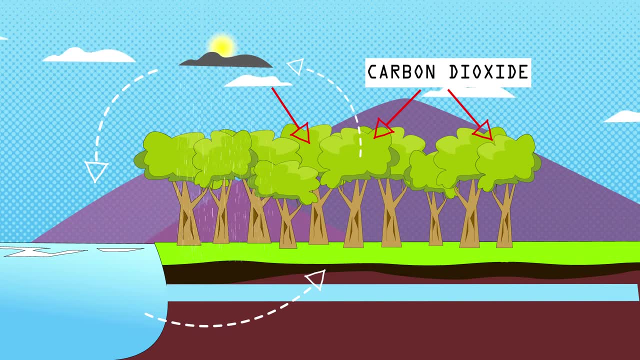 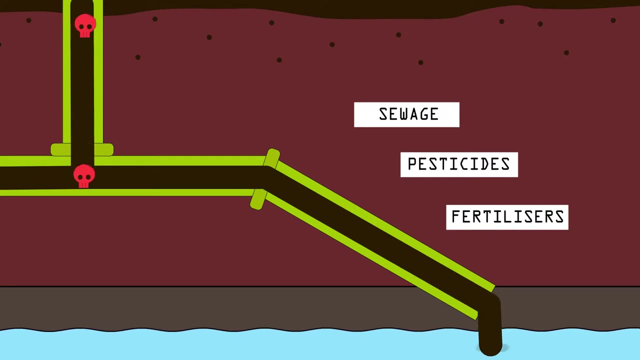 used to recycling fresh water across the globe. Trees are also able to take in and store carbon dioxide, which helps regulate the earth's temperature. As well as burning fossil fuels and deforestation, humans also create lots of waste. Sewage pesticides and fertilizers enter the water. 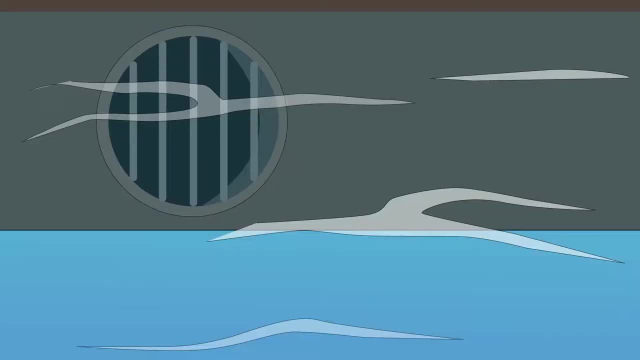 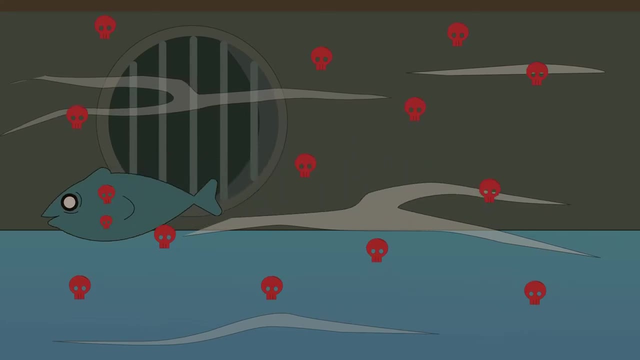 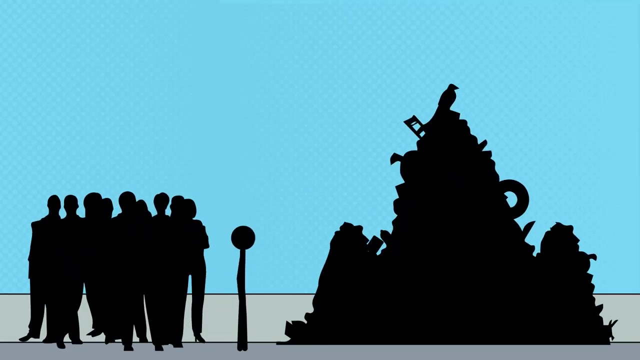 They may contain toxic substances that can kill organisms and impact on whole food webs. Pesticides can accumulate in the tissues of organisms and stay in the environment for many years. A combination of a growing population and a throwaway culture. we also have increasing 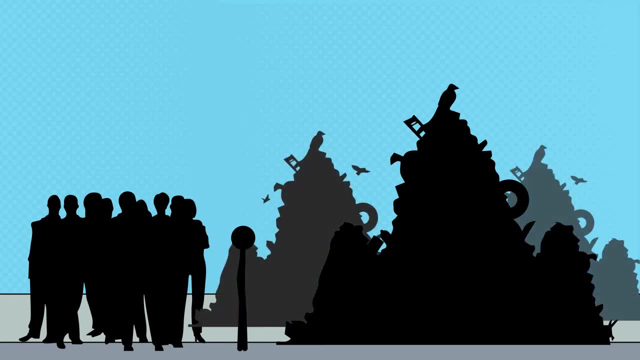 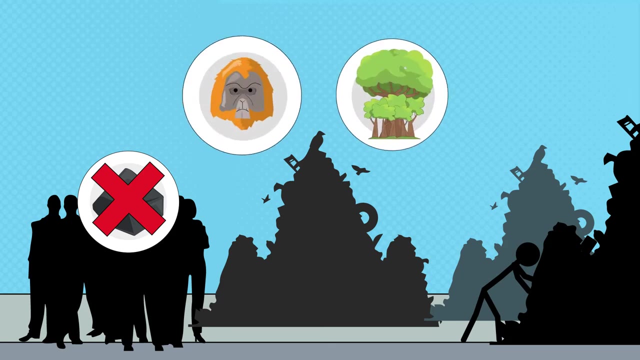 demands for dirty, wasteful landfill. But let's end on a happier note. There is some hope. People are coming to realise the impact we are having on the environment, and governments are aiming to cut down their reliance on fossil fuels and putting schemes into place to help protect forests and endangered species. 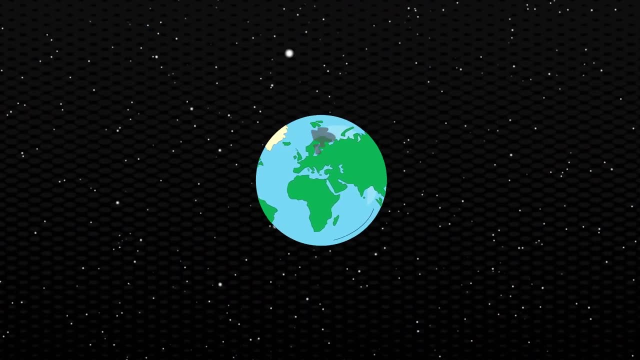 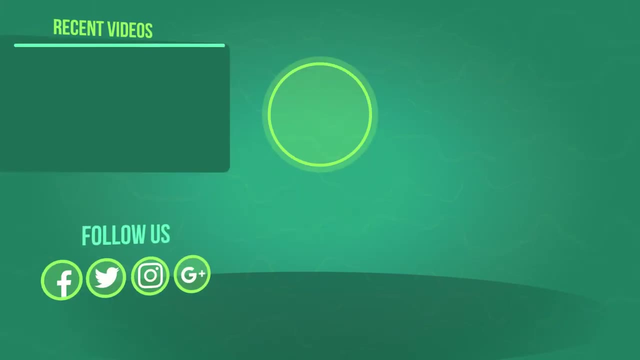 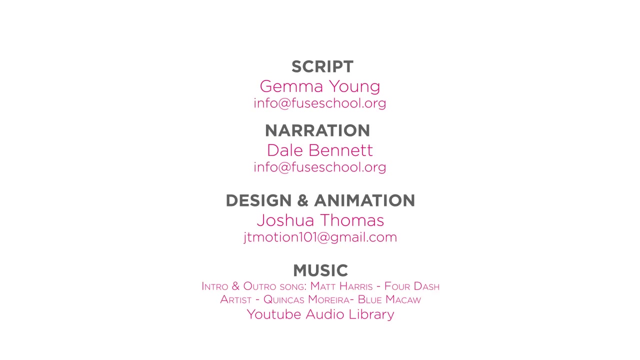 So in this video, you have learnt about how human activity has an impact on the environment. If you liked the video, give it a thumbs up and don't forget to subscribe. Comment below if you have any questions. Why not check out our Fusco app as well? Until next time. 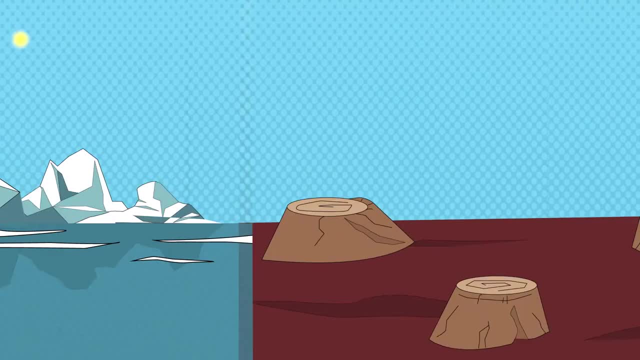 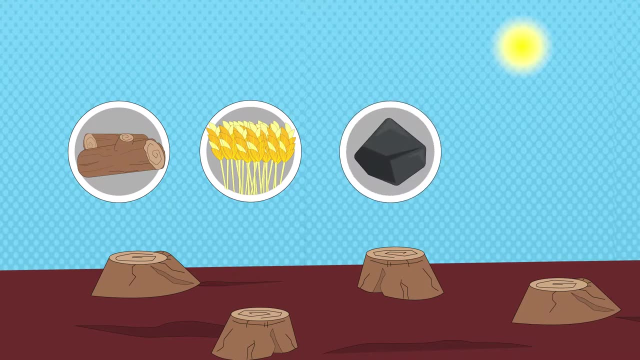 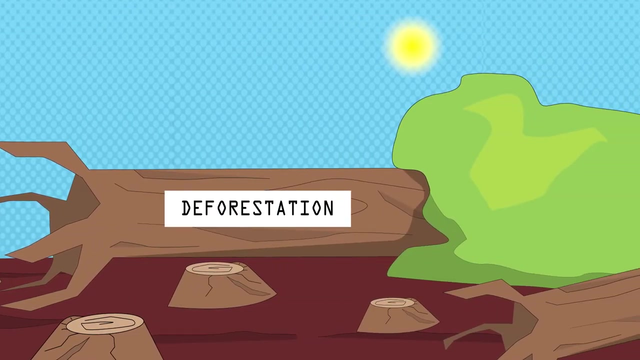 its habitat and is an endangered species. Humans also require resources. Large areas of forest are cleared to make more room for agriculture or to mine minerals or for growing other resources like palm oil. The removal of trees is called deforestation and has an enormous impact on not only the local ecosystem but the entire planet. 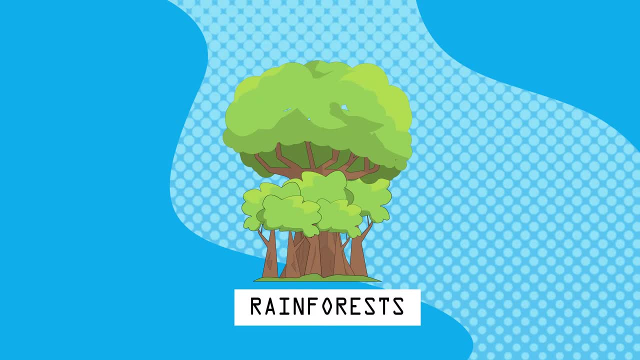 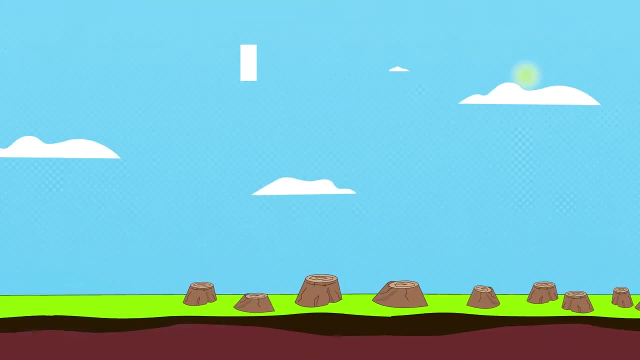 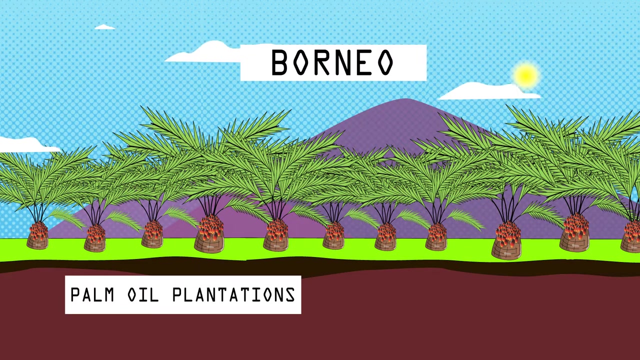 Ancient forests such as rainforests are unique ecosystems. They can support a high biodiversity and are home to species that can only live in that habitat. For example, in Borneo, rainforests are being cut down to make room for palm oil plantations. The species that live in the rainforests cannot. 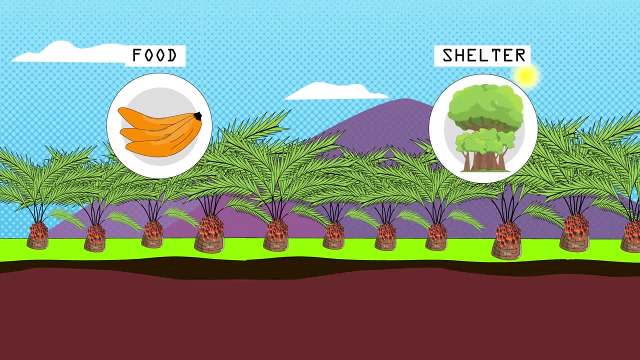 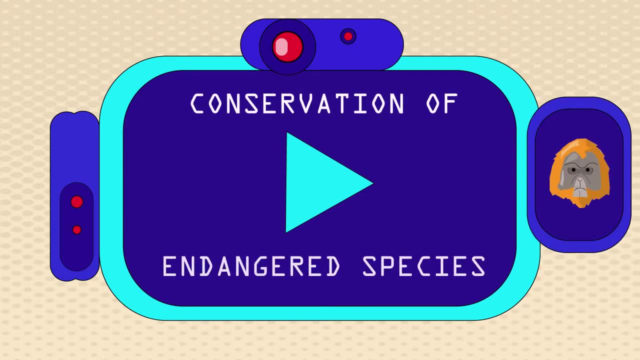 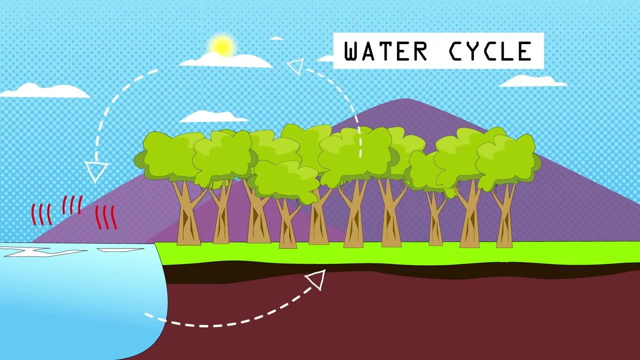 survive in the plantations. They may not be able to find food or shelter like orangutans, who are an endangered species. You can find out more about endangered species and how conservation is helping them by watching this video. Forests provide services to the planet. They are important in the water cycle, recycling, 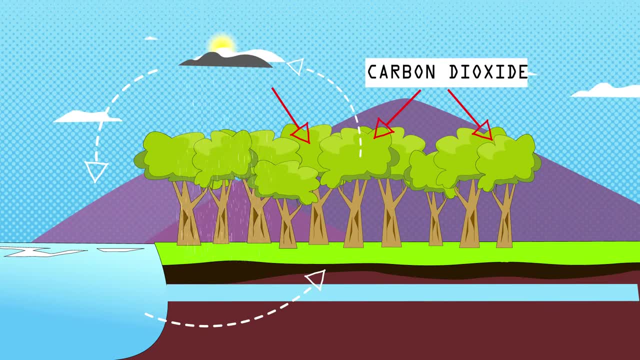 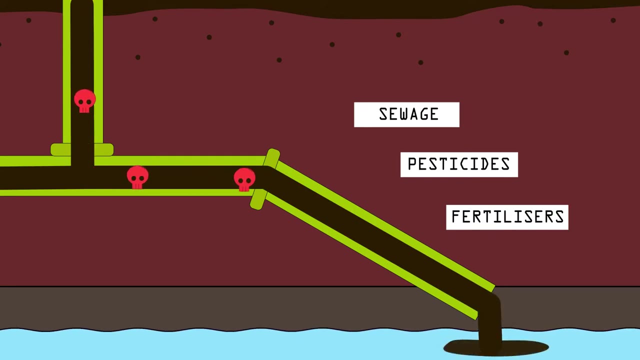 and fresh water across the globe. Trees are also able to take in and store carbon dioxide, which helps regulate the Earth's temperature. As well as burning fossil fuels and deforestation, humans also create lots of waste. Sewage pesticides and fertilizers enter the water. 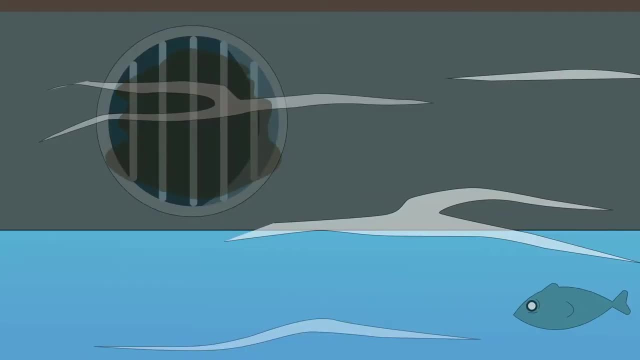 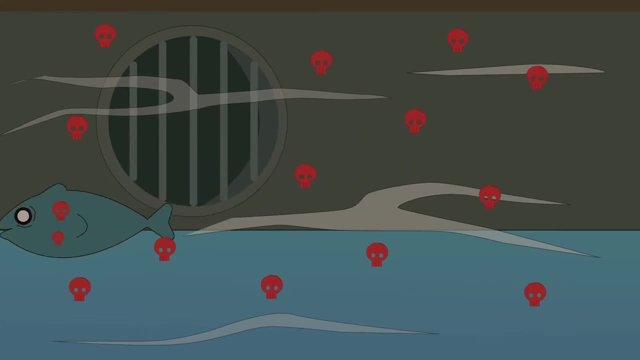 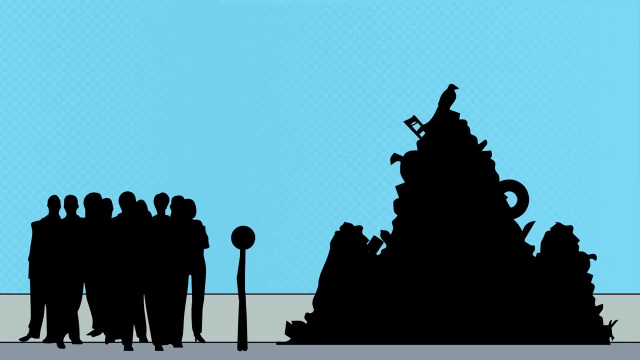 They may contain toxic substances that can kill organisms and impact on whole food webs. Pesticides can accumulate in the tissues of organisms and stay in the environment for many years. A combination of a growing population and a throwaway culture. we also have increasing 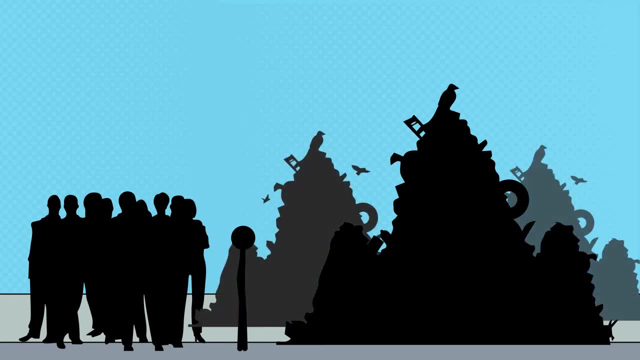 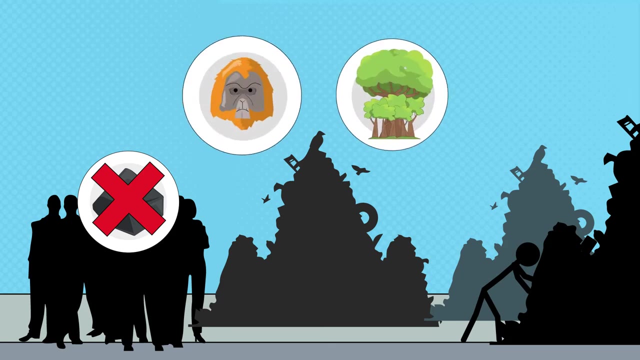 demands for dirty, wasteful landfill. But let's end on a happier note. There is some hope. People are coming to realize the impact we are having on the environment, and governments are aiming to cut down their reliance on fossil fuels and putting schemes into place to help protect forests and endangered species. 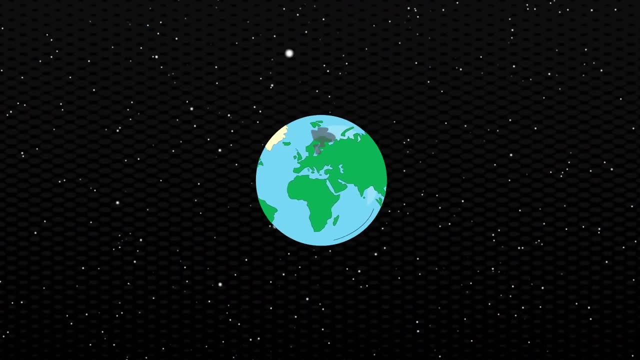 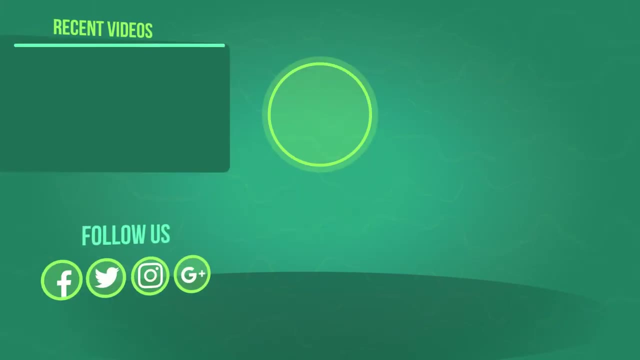 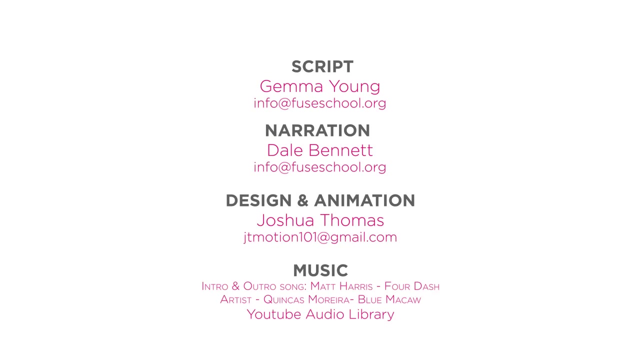 So in this video, you have learned about how human activity has a negative impact on the Earth because of burning fossil fuels, deforestation and creating waste.